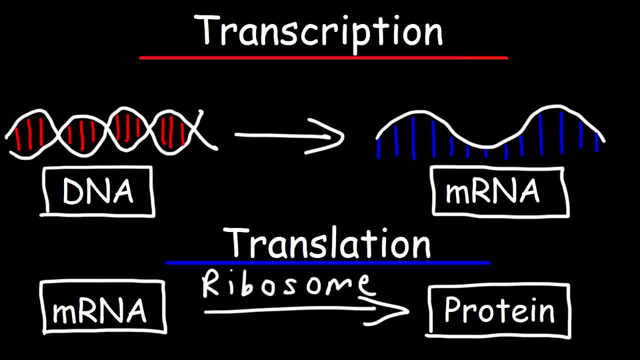 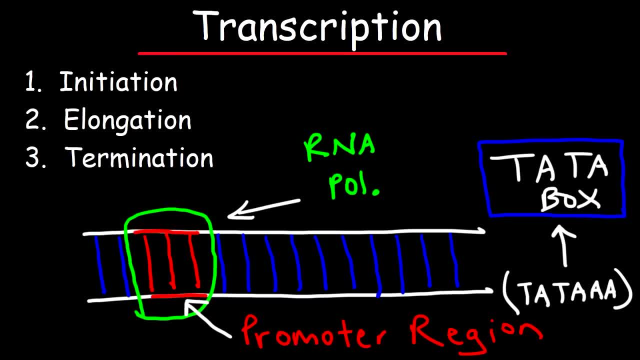 to talk about that shortly, But let's go over the ribosome. Then let's talk about transcription first, before we talk about translation. Transcription occurs in three steps: initiation, elongation and termination. Now, during initiation, RNA polymerase binds to the promoter region of DNA. 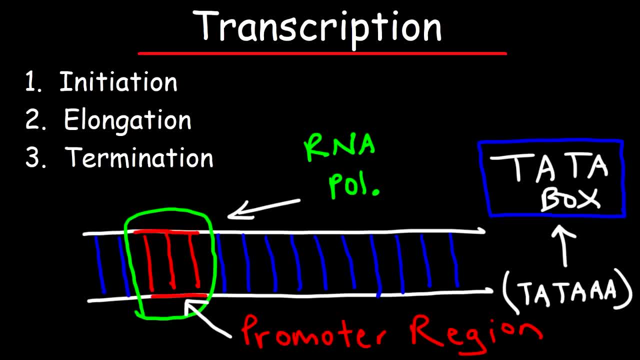 Now, what is the promoter region? The promoter region is basically a short sequence of DNA In eukaryotic DNA. it is a short sequence of Patrol DNA. It is the short sequence of DNA that binds to a promoter region. It's TATAAA, also known as the tata box. 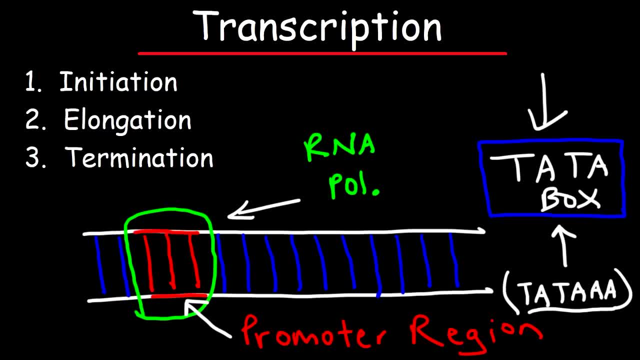 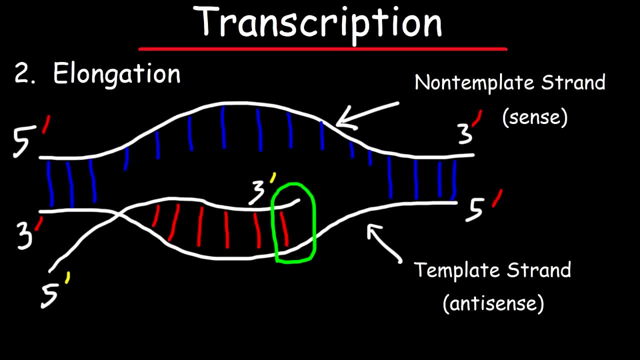 Now this sequence is located 25 nucleotides upstream of the site where transcription begins. The next thing that RNA polymerase does is it causes the two DNA strands to separate And during elongation it begins to add nucleotides to the growing mRNA strand that we see here. 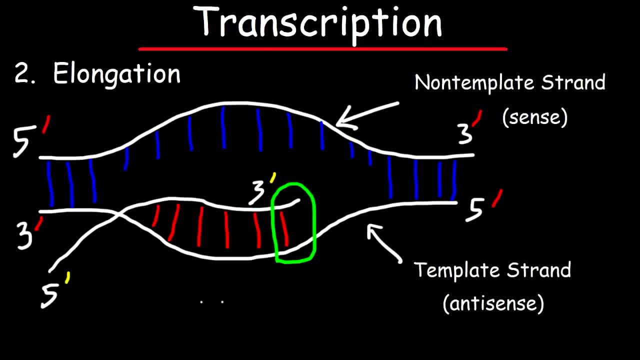 Thus, RNA polymerase synthesizes mRNA, starting from the 5' end, going to the 3' end. However, RNA polymerase, it reads the DNA strand into 3 to the 5'. Now there's two strands that you need to be familiar with. 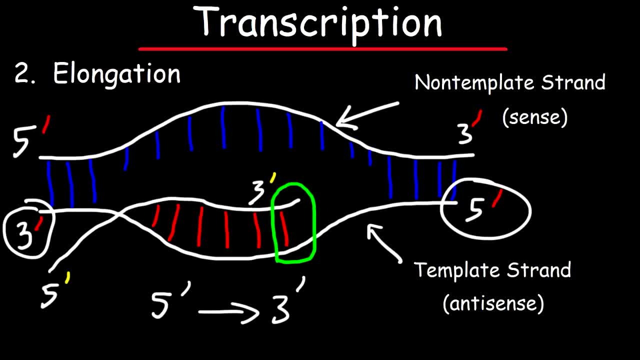 The first one, the one that's used to synthesize mRNA, is called the template strand or the antisense strand, So that's the one in which RNA polymerase is active. upon The other one, which is not used, this is called the non-template strand, also known as the sense strand. 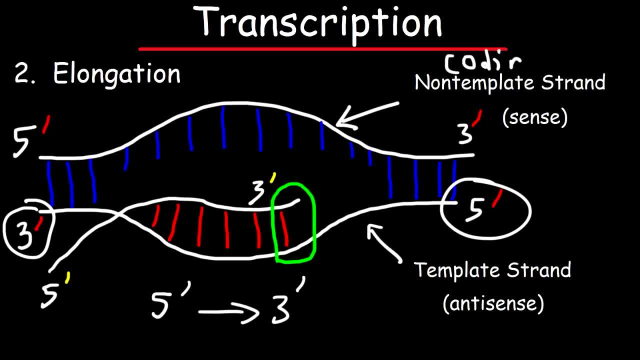 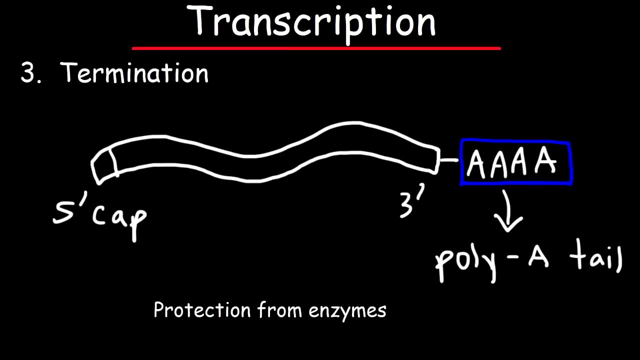 Some textbooks will call it antisense. The coding strand, because its sequence matches up with RNA, except the fact that uracil is found in RNA but thymine is found in DNA. Now, during the last step of transcription, which is the termination step, the RNA polymerase molecule. the mRNA strand. they all separate from the DNA template strand. 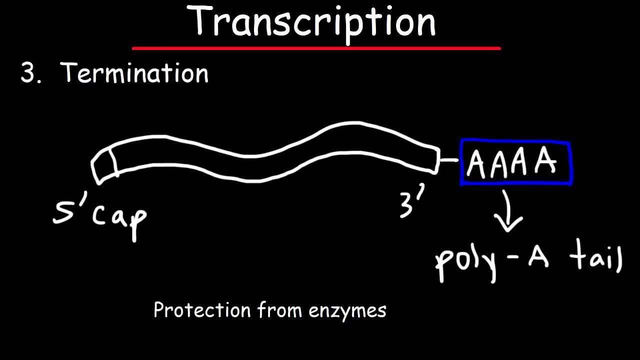 Now in this step, the poly-A polymerase enzyme. it caps the 3' end of the mRNA strand and this is known as the poly-A tail. Now also during the beginning of transcription, the 5' end is also capped. 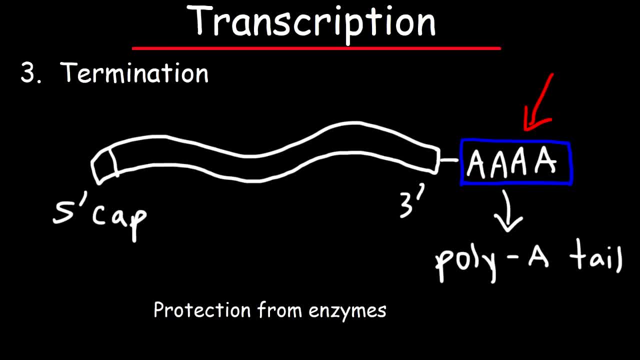 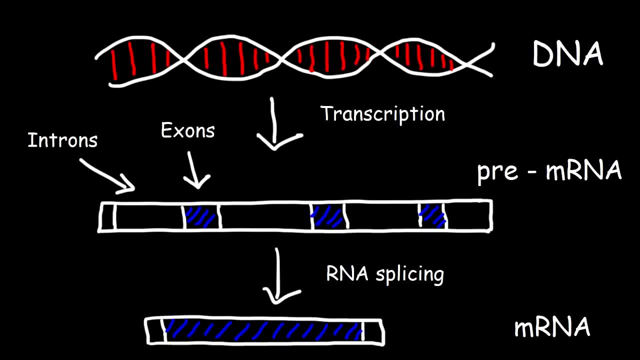 And the reason for this is to protect the mRNA strand from being degraded by certain enzymes At the end of the termination step during transcription. DNA DNA- DNA DNA- has been used to create a pre-messenger RNA strand. Now this particular strand has something known as introns and exons. 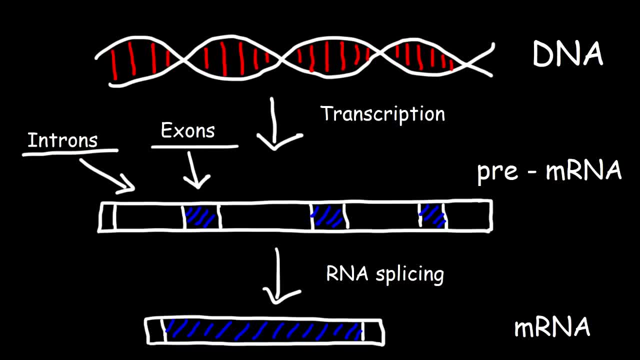 Introns are basically longer sequences of nucleotides that do not code for anything. So these they must be removed in a process known as RNA splicin. Now the exons. the exons, those are shorter sequences of nucleotides and they're going to be used to synthesize proteins. 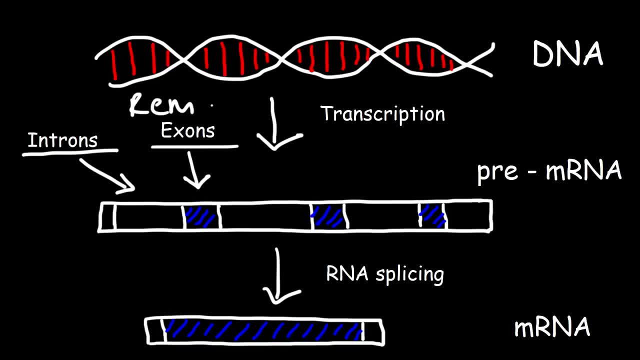 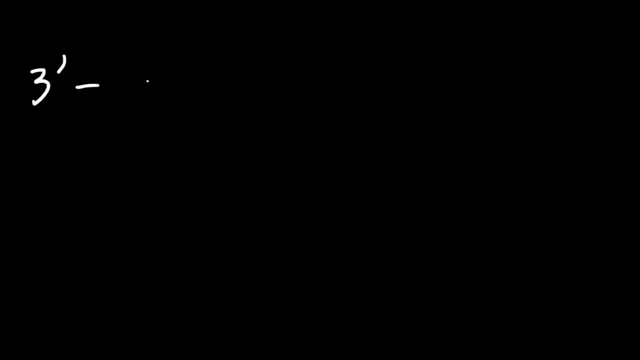 And so the exons remain, but the introns, they must be removed. And so now we have a completed messenger RNA strand. Now let's work on a practice problem. Let's say, if you're given a sequence of of nucleotides on a DNA strand and you're asked to write the correspondent, 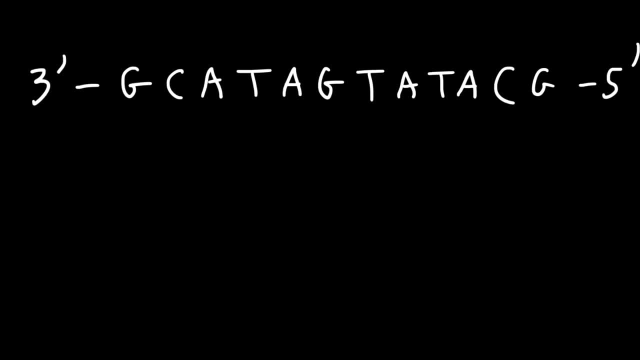 sequence on an mRNA strand. what would it be? feel free to pause the video and try it. so if we're reading the DNA strand from the three to five direction, we're gonna have to write the correspondent mRNA sequence in the five to three direction. so what letter corresponds to G? it's important to know that gene. 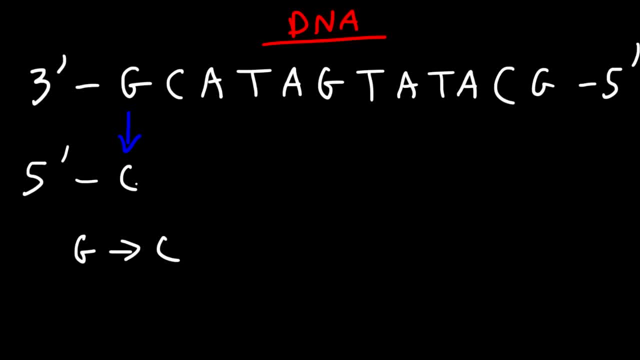 always corresponds to C, and vice versa, C corresponds to G. now, what letter corresponds to a? a usually corresponds to T, but there's no T and RNA. instead, a is going to correspond to you for yourself, but T and DNA corresponds to a in RNA, and so if we continue, 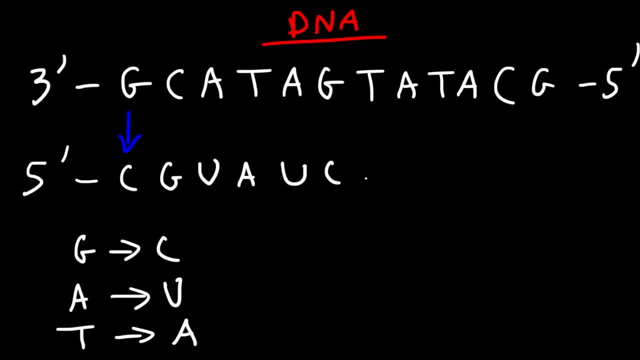 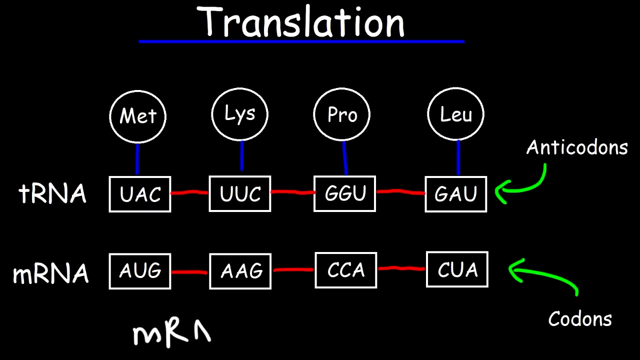 everything else is going to be: you see, a, you, a, you, gc. and so this is the mRNA strand that corresponds to the nucleotide sequence in DNA listed above. now let's talk about translation, which is the process of taking the information stored on an mRNA strand, and 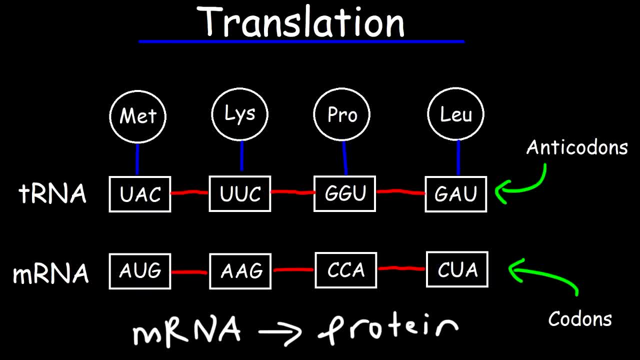 using it to construct a protein. so once the mRNA strand is synthesized in the nucleus, it leaves the nucleus and enters the cytosol, where it interacts with a free ribosome or one that is attached to the rough ER. now, within the ribosome, it's going to interact with a tRNA molecule or a transfer RNA molecule. 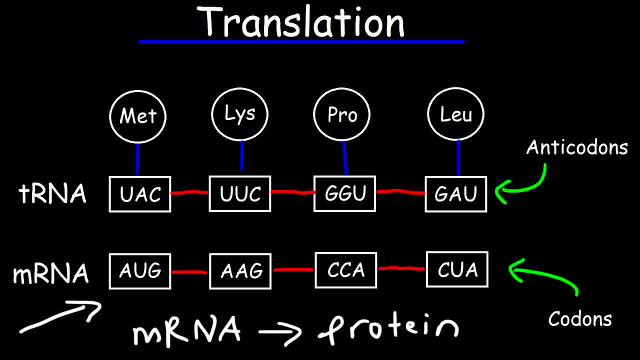 now let's focus on the sequence of nucleotides on the mRNA strand. notice that they're separated in sets of three. each set of three nucleotides represents a code on which matches up with another three nucleotides on the tRNA molecule, known as an anti code on, and each code on matches up with a specific amino acid. 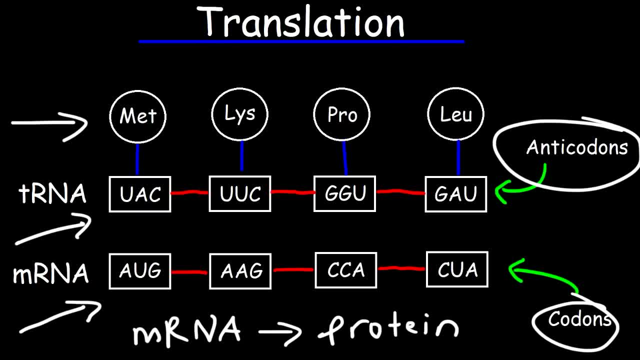 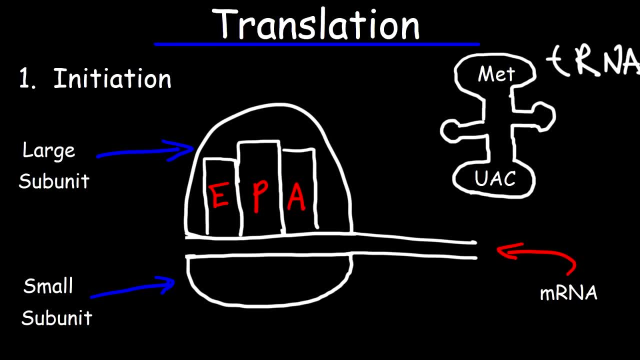 and so that's how the information stored in the mRNA strand can be used to construct a specific protein. We're going to talk more about this later in this video. Translation, like transcription, occurs in three steps: initiation, elongation and termination. So here in this picture we have a ribosome which is 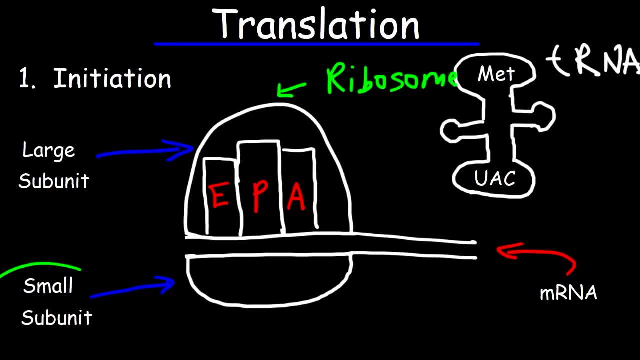 composed of two subunits- the small subunit and the large subunit- and the ribosome has three active sites: the E site, the P site and the A site. Now, during initiation, we have the start codon AUG, which corresponds to the anticodon UAC. 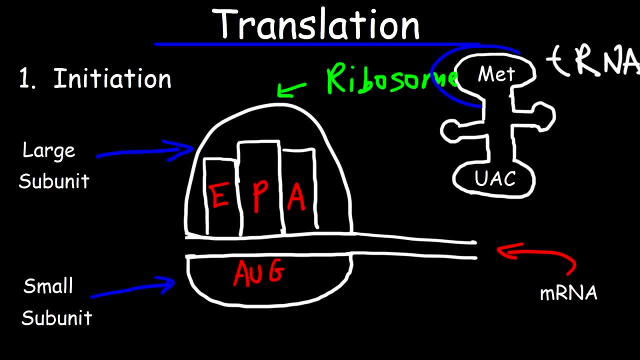 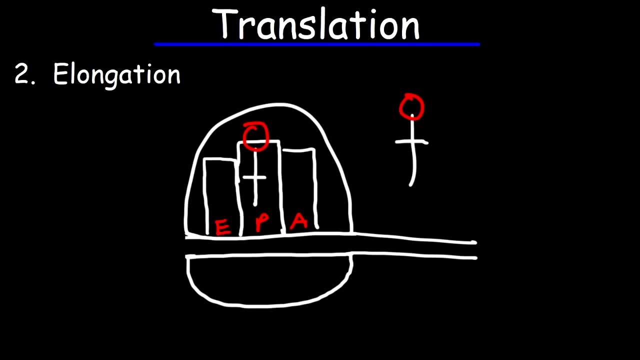 Now that particular tRNA molecule has the methionine amino acid attached to it and this tRNA molecule, it enters the ribosome at the P site, also known as the peptidyl site, where the peptide bonds are formed. Now, during the second step of 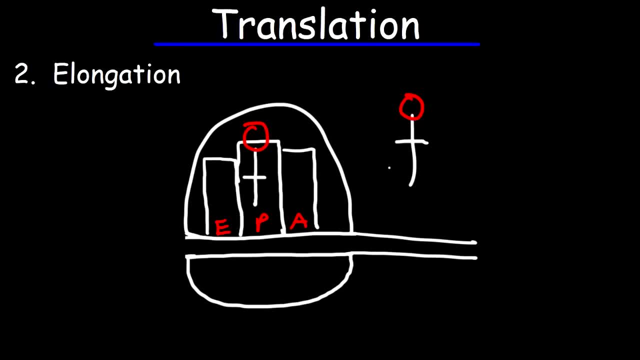 translation. that is, during elongation, another tRNA molecule enters the A site- So I'm just going to draw it here- and during that process a covalent bond will form between the two amino acids and the peptidyl, And when it's born, the pro emperor ends up getting new amino acids that we see here. 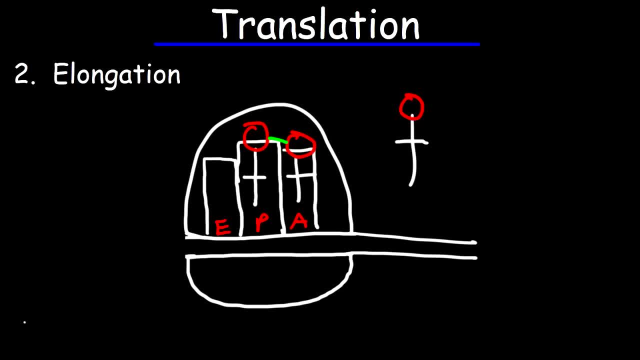 highlighted by the red circles. now, as the process continues, the tRNA molecule in the p-site we'll move to the E site, and as it does so, it's going to lose an amino acid, and so what's going to happen is we're going to have a growing chain. 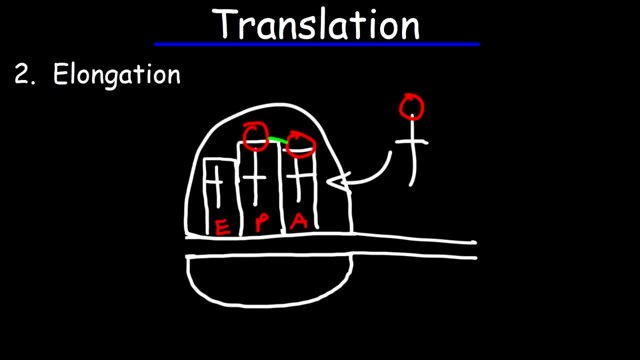 of amino acids that will leave or extend out of the ribosome. so make sure you understand at that. tRNA molecules: they enter the A site and then they exit until the antס2 gets into the P site from the E site And in the process the amino acids are being joined together. So over time 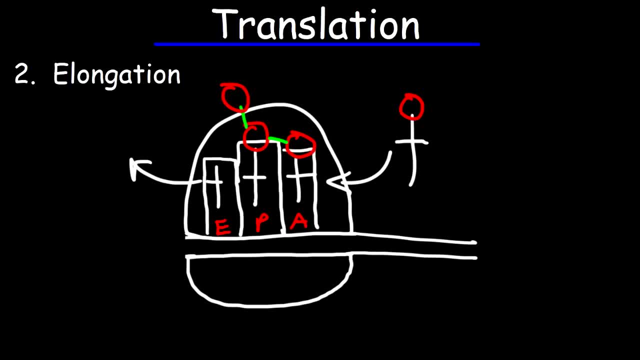 this polypeptide chain is going to grow, creating a protein. The last step of translation, the termination step, begins when a stop codon is read. Now there are three stop codons that you need to be familiar with. The first one is UAA. 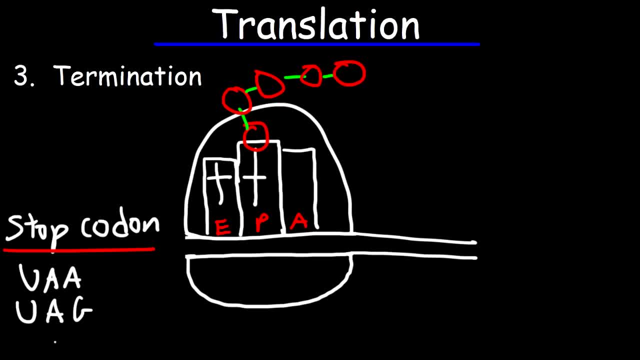 and then the second one is UAG and the third one is UGA. Now these stop codons, also known as nonsense codons. they don't code for any specific tRNA molecule. Instead, when these are read as the A site, 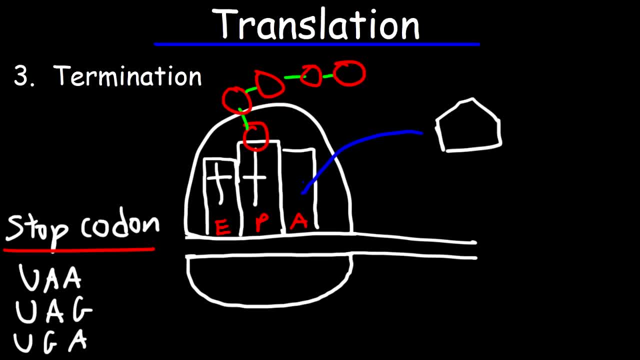 they cause a release factor to enter the A site, which causes the small and the large ribosomal subunits to basically disassemble. So this is where translation ends and the protein it leaves the ribosome where it eventually goes to the Golgi body. 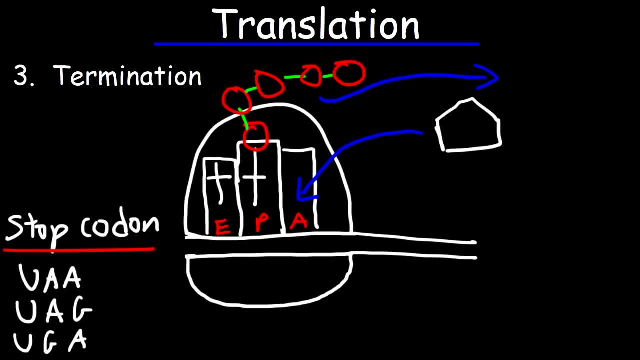 for further processing and modification. At the Golgi body, the proteins undergo folding, where they form a specific shape to perform a specific function, And that's basically it for this video. Hopefully it gave you a good overview of transcription and translation. So that's all I got. Thanks for watching.